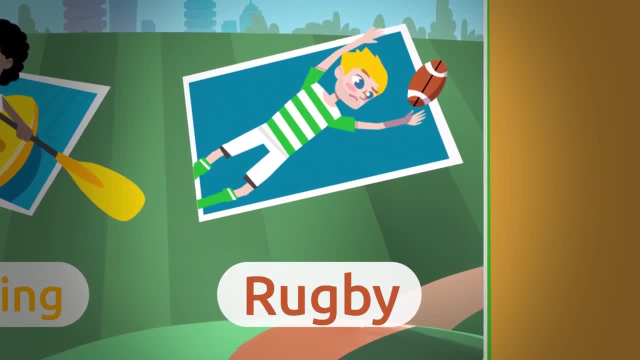 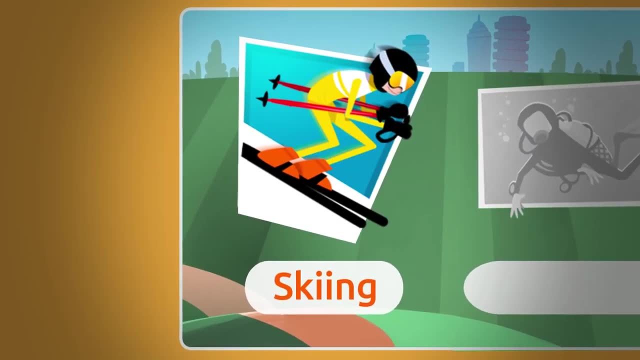 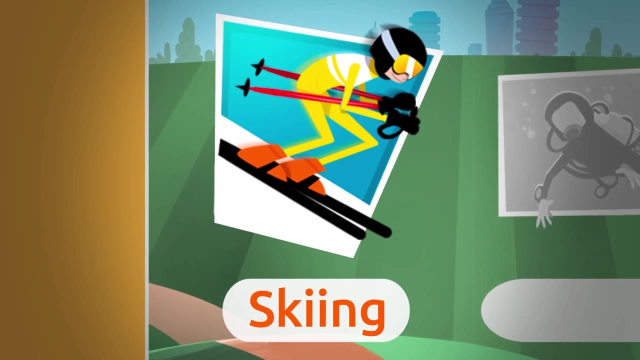 The ball is oval-shaped Rugby. Let's see this next one, A skiing sticker To ski skiers slide on snow using skis that are long boards fixed on their feet Skiing. And the last sticker is a scuba diving sticker. 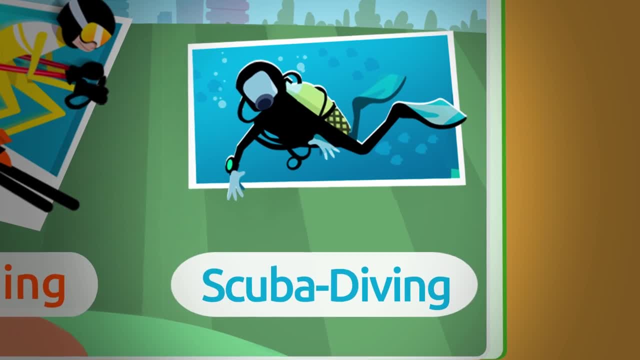 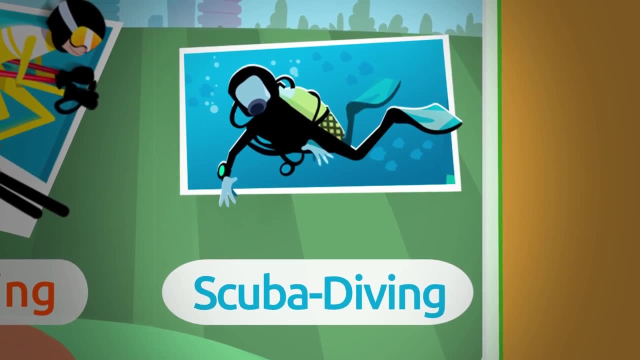 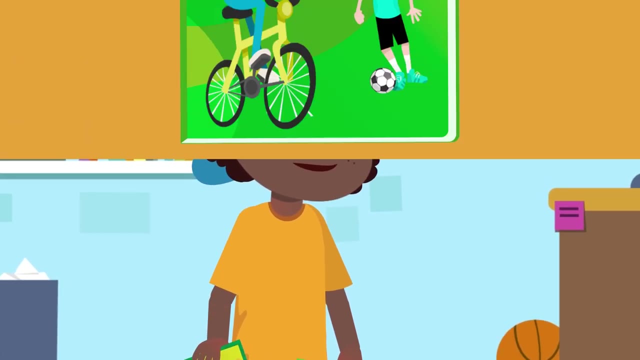 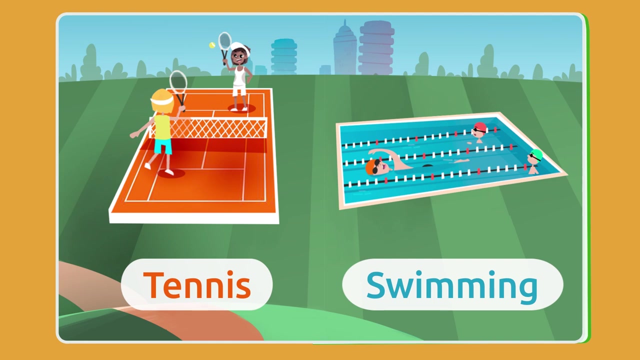 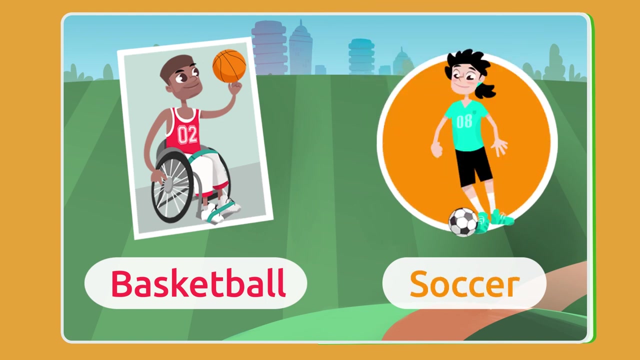 Scuba diving is practiced underwater. You use goggles, diving flippers and a diving tank. Scuba diving. We learned so many sports words today. Shall we recap them: Tennis, Swimming, Basketball, Soccer, Soccer, товzetmeerscom. 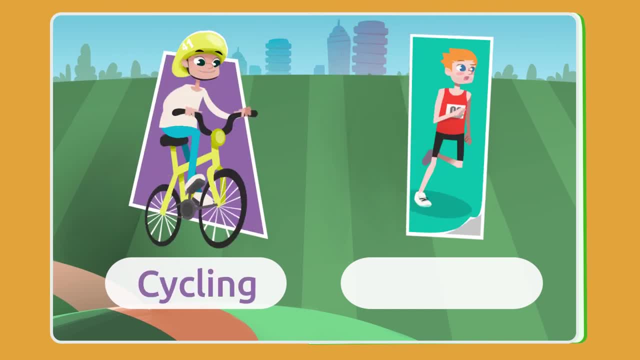 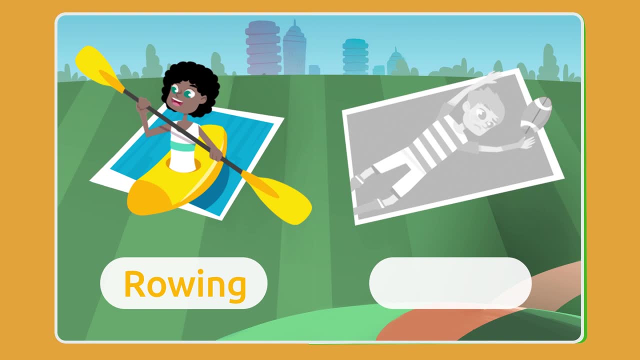 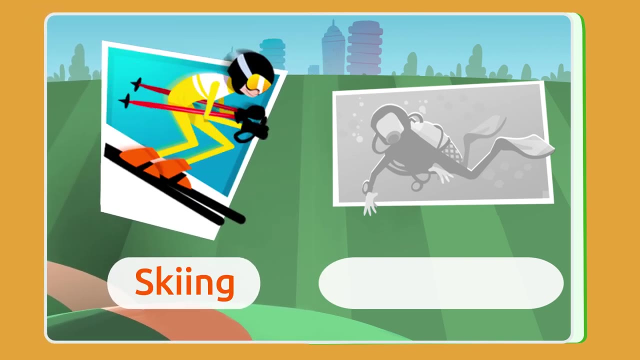 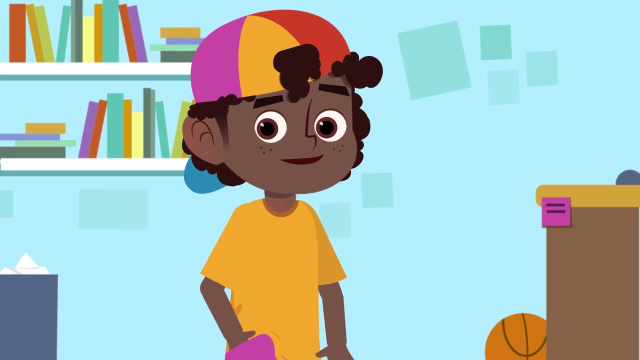 Cycling, Fishing, Athletics, Fitness, Cycling, Sports Athletics: Ronin 將imientos, aeda Wrestling Gym Sport James Skiing, Hockey Skippings. veland, Scuba diving. Scuba diving. 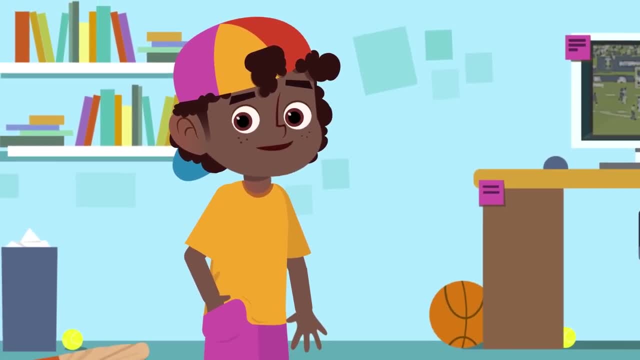 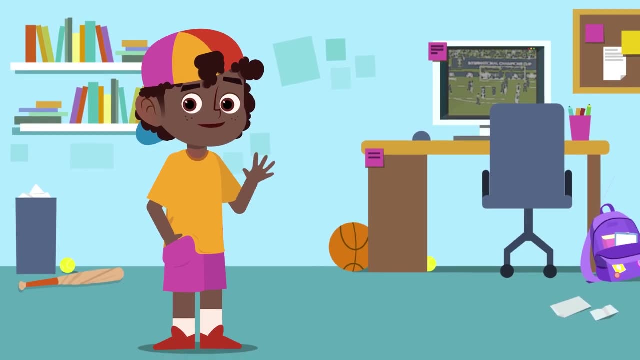 How amazing. Well, I still have to finish putting the stickers in the second part, in the second part of the album. Don't miss the next video to learn more sports words. See you soon. Hello again, friends. We have to complete the sports sticker album. 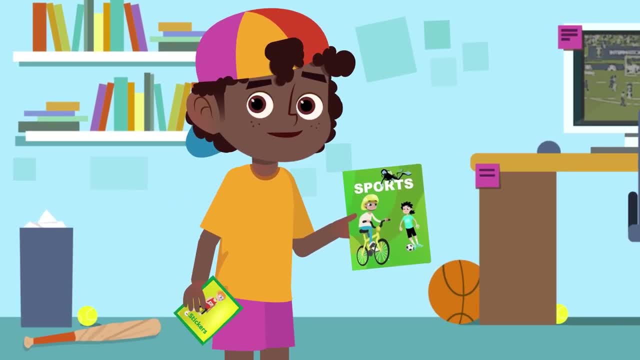 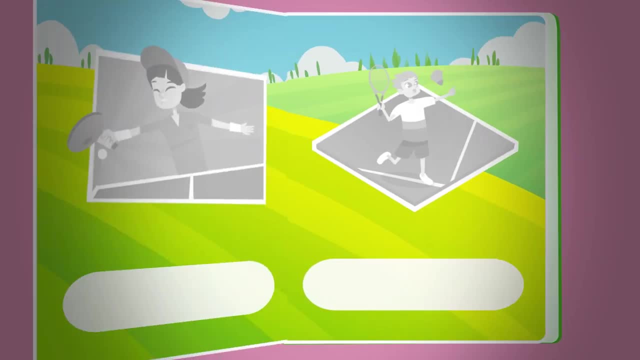 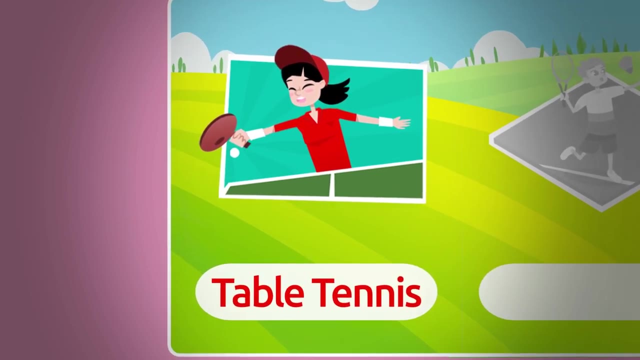 we started in the previous video. I have another envelope with stickers. Let's see which ones I got this time. The first sticker is a table tennis sticker. To play table tennis you need a paddle, a very light ball, a table. 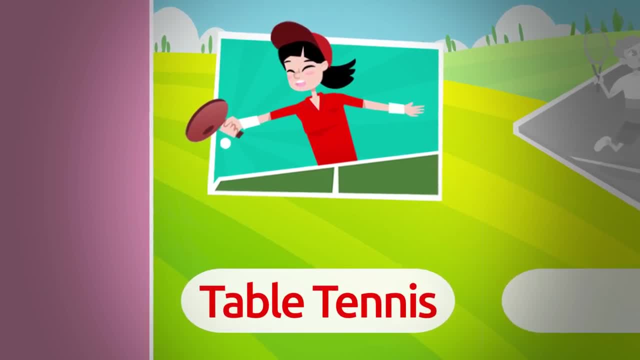 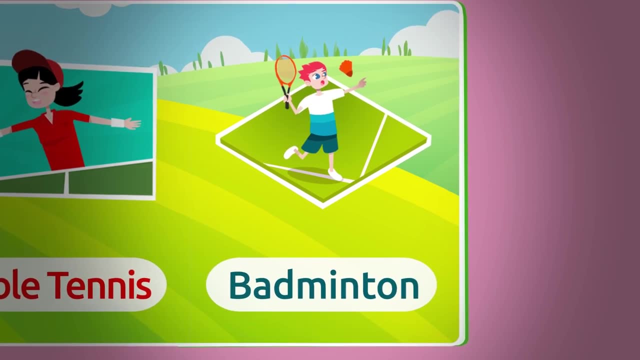 and a net. Oh, You also need an opponent Table tennis. The next one is a badminton sticker. Badminton is very much like tennis. It's a racket sport too, But instead of a ball you hit the shuttlecock. 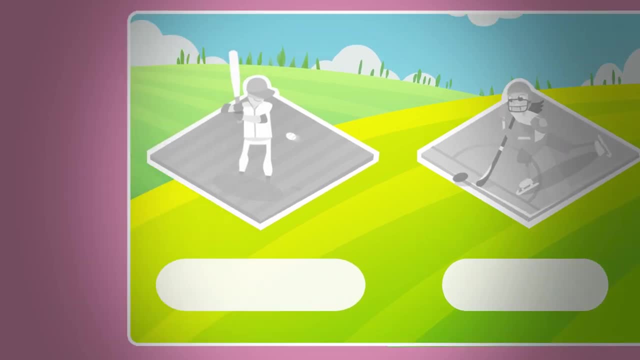 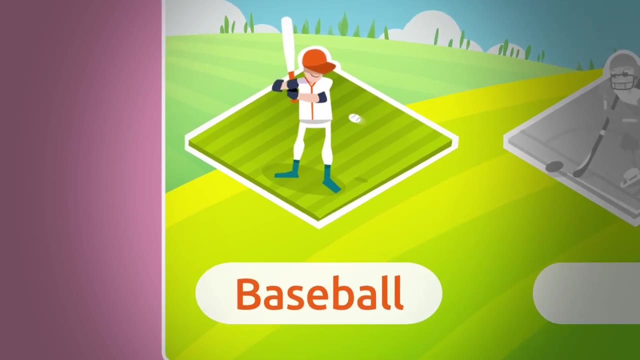 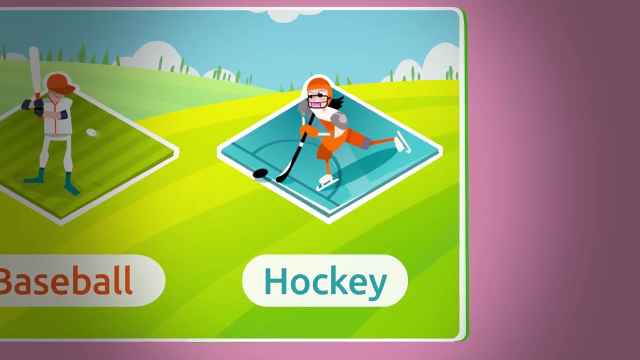 Badminton And this one is a a baseball sticker. In baseball, players use the baseball bat to hit the ball thrown by the opponent Baseball. This is a hockey sticker. To play hockey, you need to shoot the puck or the ball. 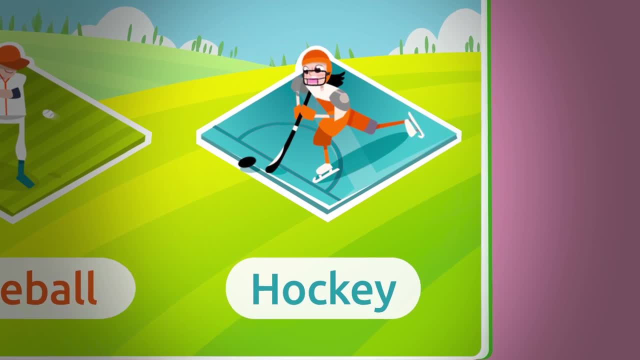 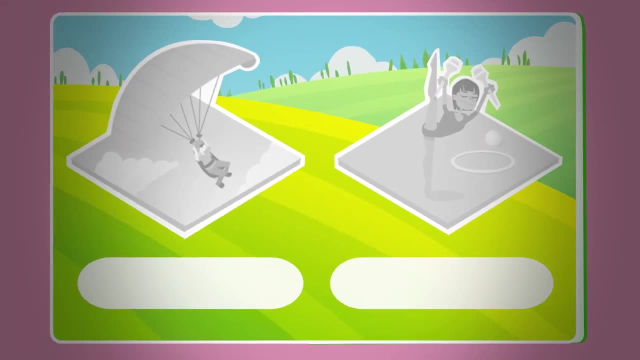 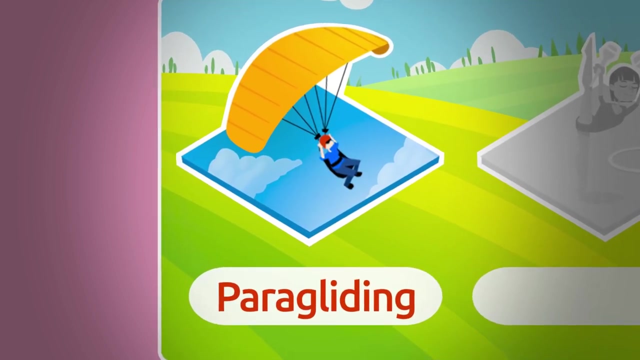 into the opponent's goal. using just a stick, You can play hockey on ice, grass or turf fields Hockey. Let's have a look at the next one: Paragliding. Paragliding consists in soaring from a slope using a parachute. 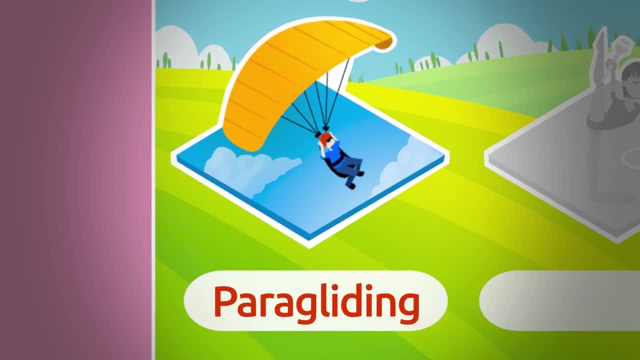 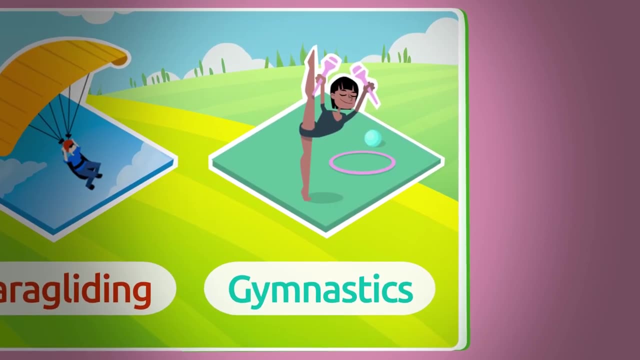 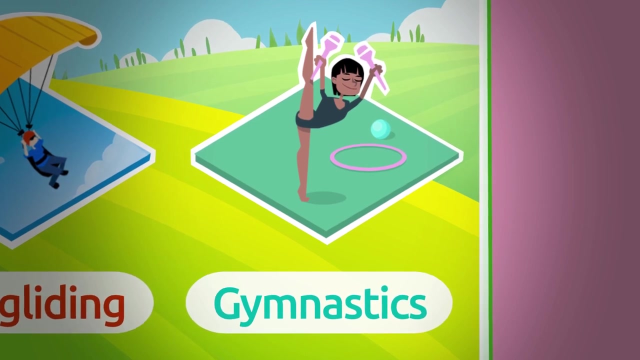 to control the descend Paragliding. Let's see what we have here: Gymnastics. Gymnastics is a sport based on a set of exercises to develop and improve balance, agility, flexibility or resistance Gymnastics. 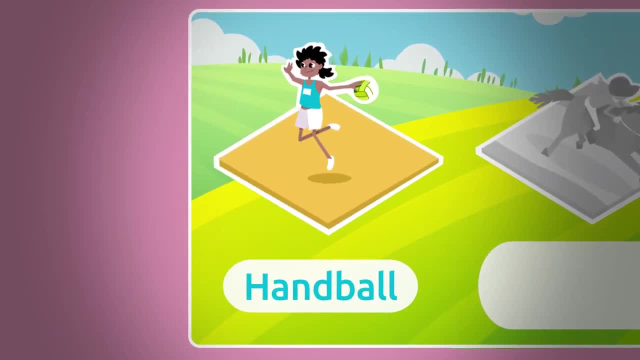 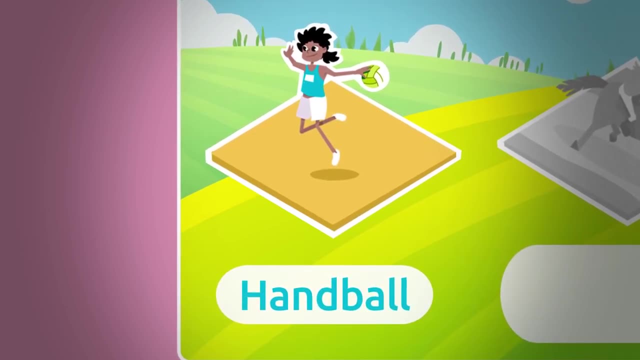 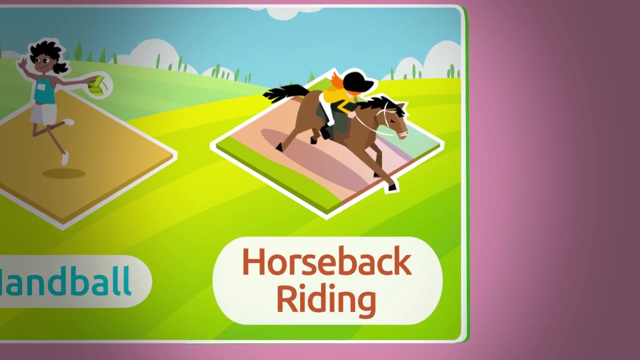 The next sticker is a handball sticker. Handball is a sport in which the ball is shot into the opponent's goal using only your hands. Handball And this is a horseback riding sticker. Horseback riding is the sport of riding horses. 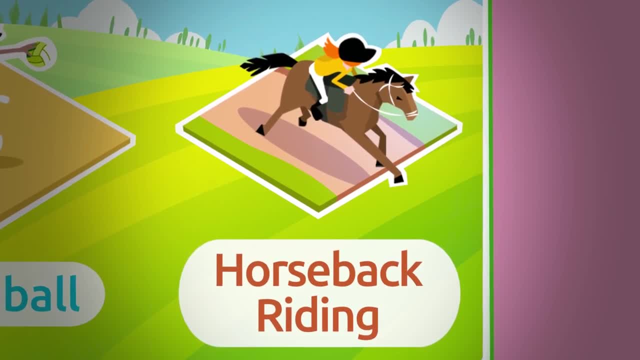 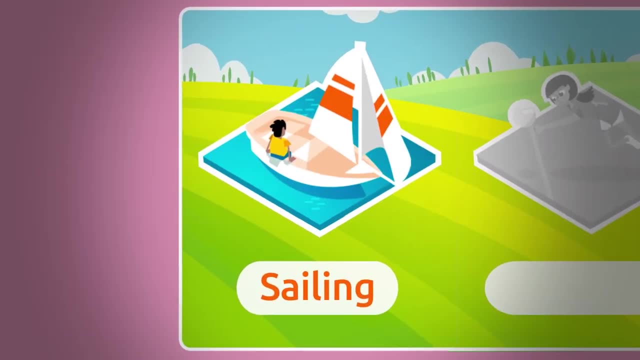 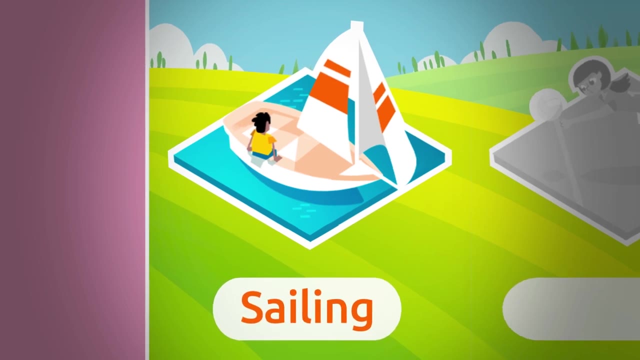 Some examples are horse racing or hurdling Horseback riding. Let's see what. the next one is A sailing sticker. Sailing is the sport of steering a sailing boat propelled by the wind Sailing. And the last one is a volleyball sticker. 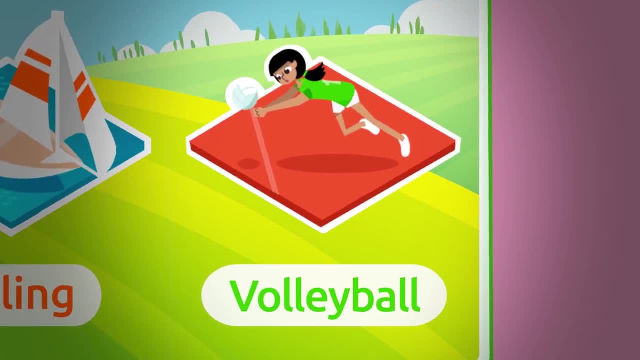 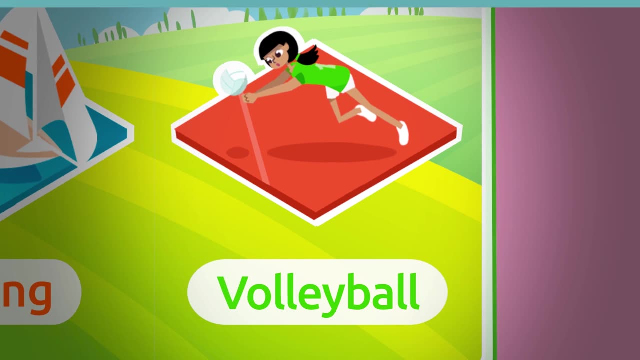 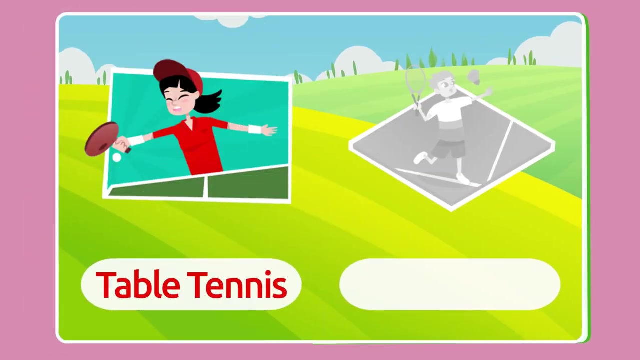 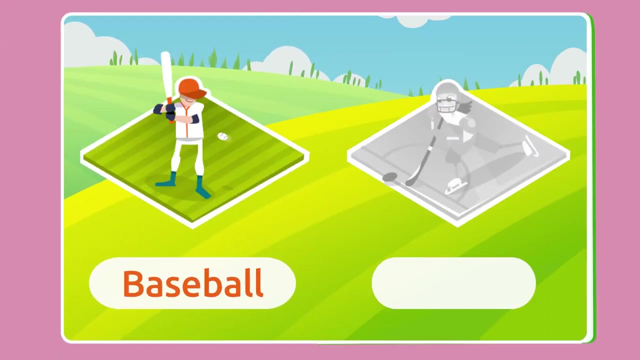 Volleyball is a team sport in which you hit a ball over the net into the opponent's court using your hands. Volleyball- So many sports. Let's recap them: Table tennis, Badminton, Baseball, Baseball, Baseball, Baseball. 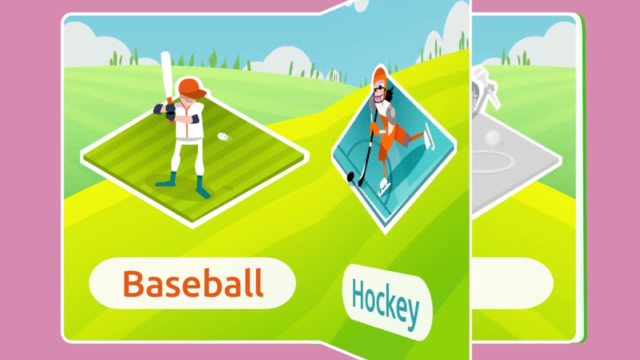 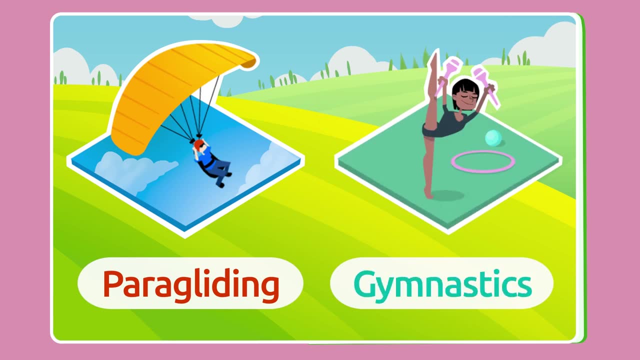 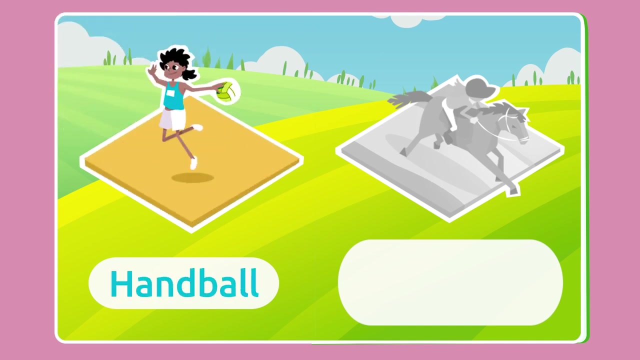 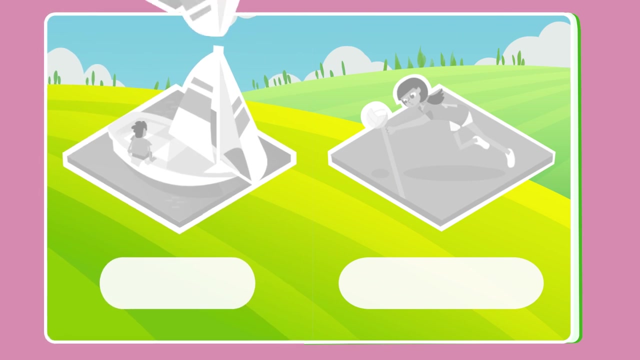 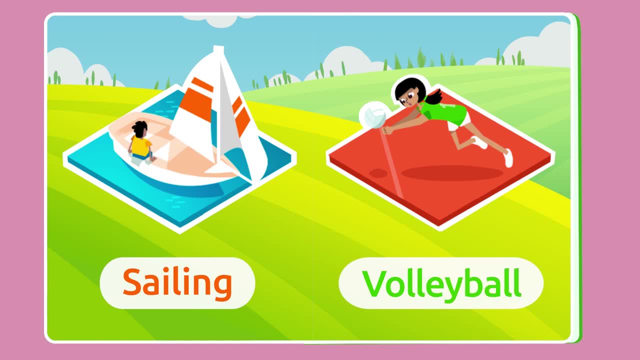 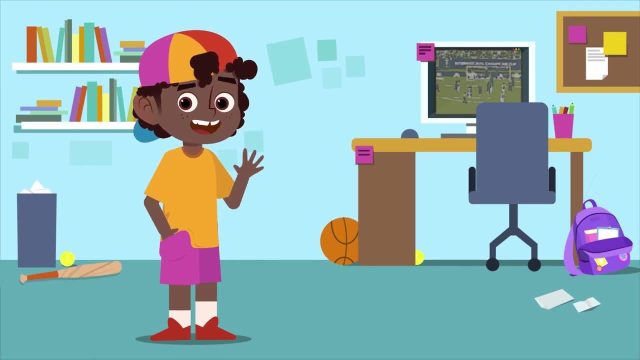 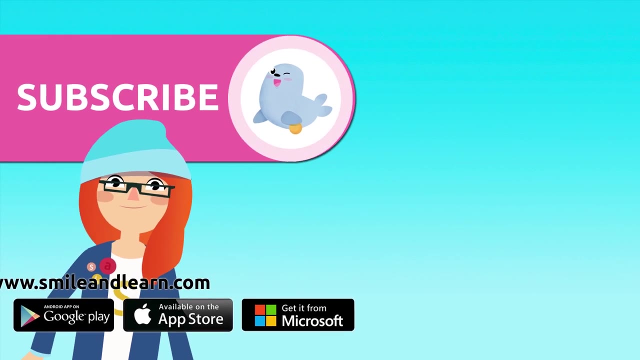 Volleyball- Awesome. We've completed the sports sticker album. Thank you for helping me. See you soon. Subscribe by clicking on the seal Ah, and if you want to keep watching more videos, click on the boxes.